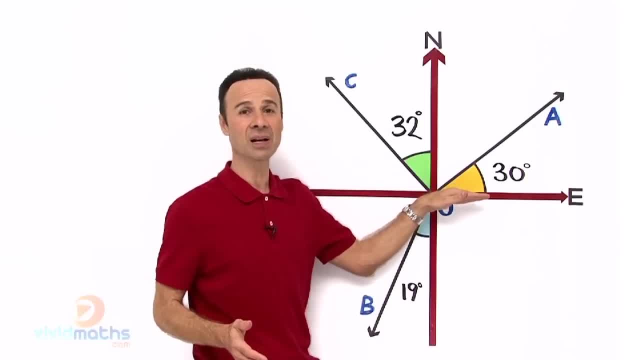 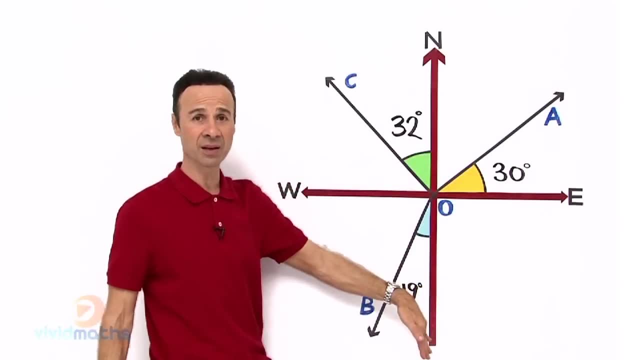 here we have a random angle, 30 degrees from the eastern bar, so you can see the eastern bar is going up here 30 degrees, so that is kind of random. and then over here we got the 180 bar down the bottom, which is the opposite of north down south, and we got 19 degrees. 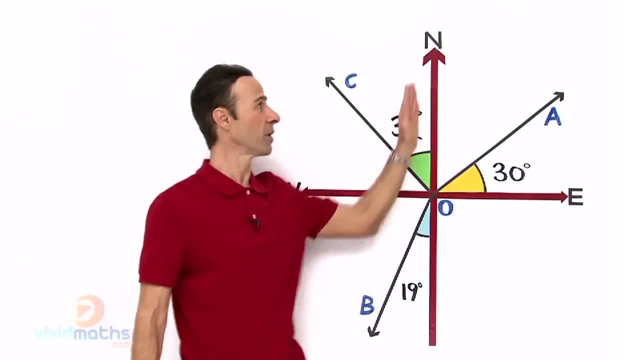 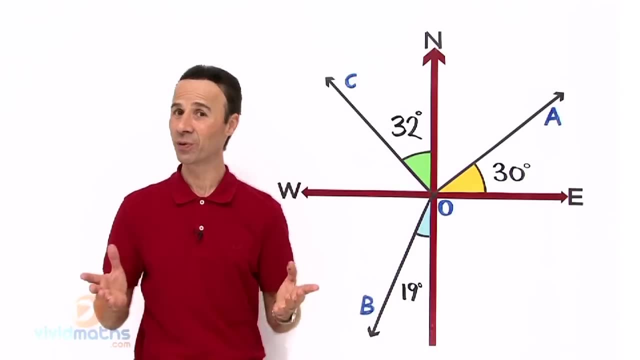 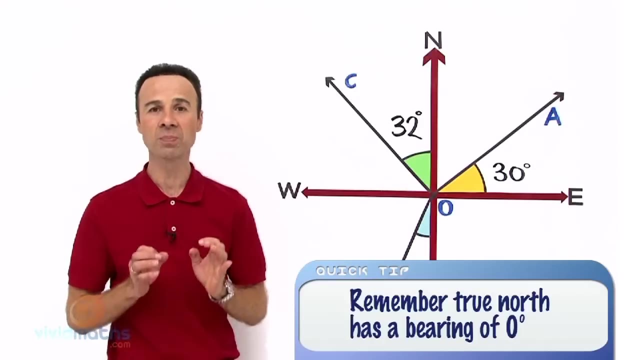 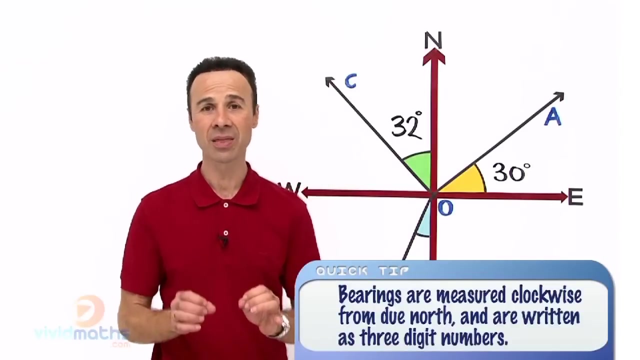 sweeping across here and then finally we have here, from the north bar backwards, anti-clockwise 32 degrees. Our mission: transform them into beautiful bearings. Now, what is that one concept? The one concept is: always begin at north and go clockwise. always begin at north and go clockwise, because nothing happens in bearings without north. 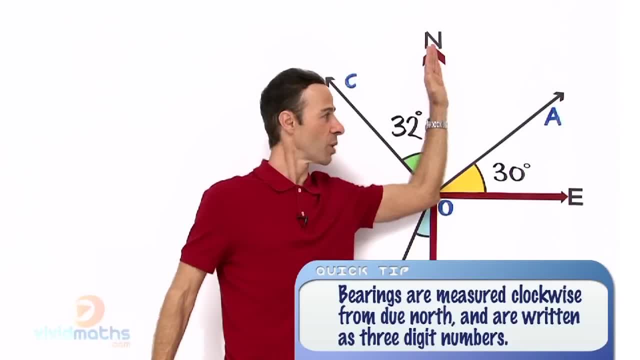 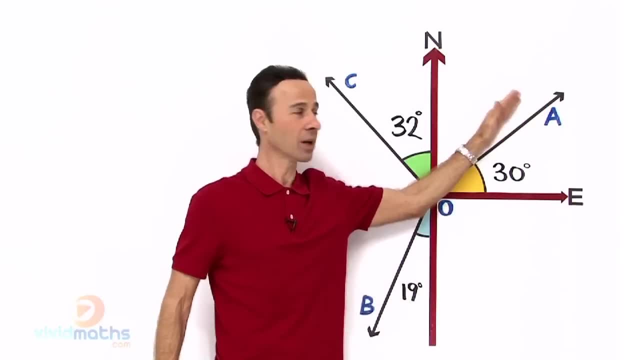 Nothing happens in bearings without north. Here is our north. we are going to take the first one and we are going to get the bearing right there: O, A from O to A bearing: first bearing. Second bearing. Third bearing. Third bearing, Fifth bearing: 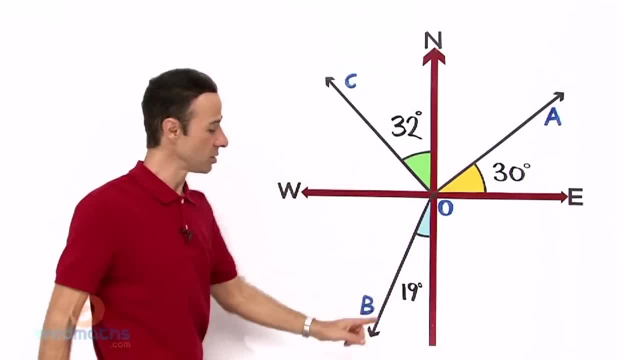 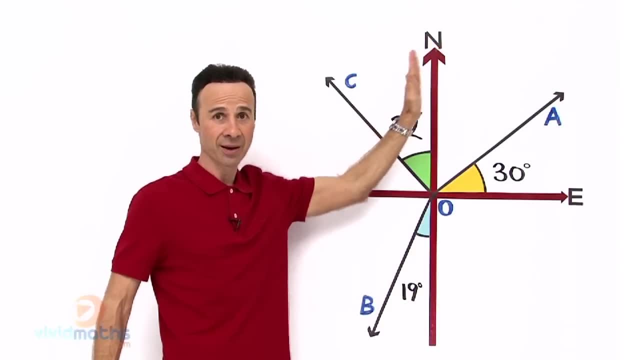 Fifth bearing, 度 And double bearing. The third one goes clockwise, sweeping all the way across to 19 degrees from north, that way from O to B And then finally, starting at north, going all the way around. almost a revolution, which is 360 degrees, going back here and by 32 degrees. 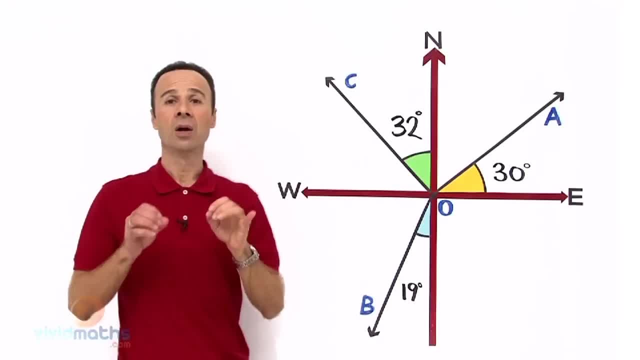 So let us go through this now. remember the concept is: no bearing can happen without north. so let us sweep through and do them all, one at a time. so the first one is right hereWe want to get the bearing right here. So the first one is right here. you want to get the bearing right there. 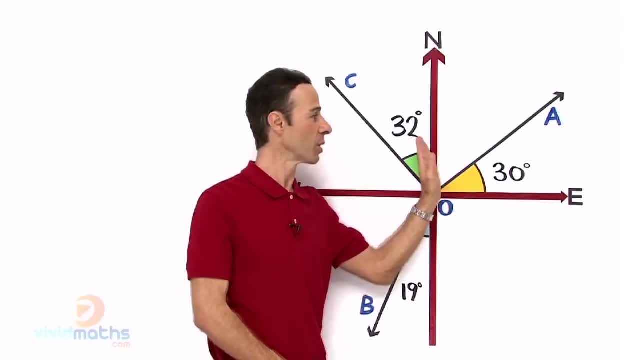 Then you go from here and now along the way, Then we go from here and then from there and now along the way. So the first feeling issung to the right. then you are going to get the bearing plus north. We want to get the bearing here. so let me mark out the bearing that we are going for. 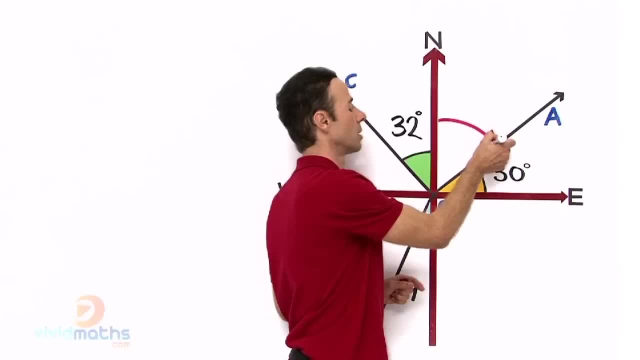 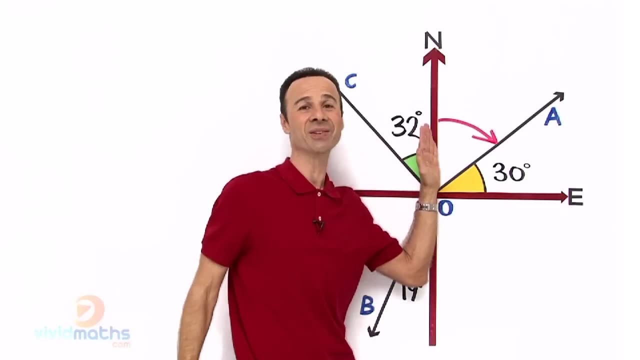 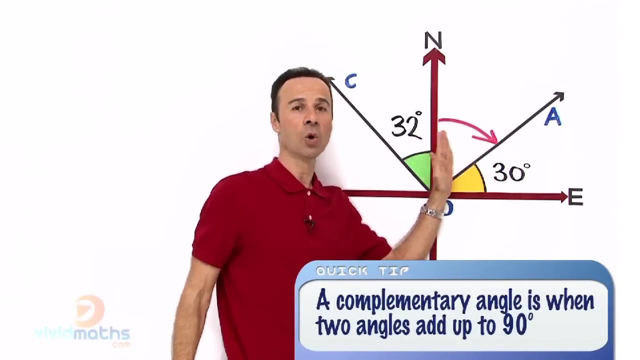 so you can see it visually – there is our first bearing. okay, that is what we are going for Now. in order for us to do this, I wonder whether you can recognize and realize, looking here, that this is complementary. So if we have 30 degrees in here, what is left over up here will give us the bearing from. 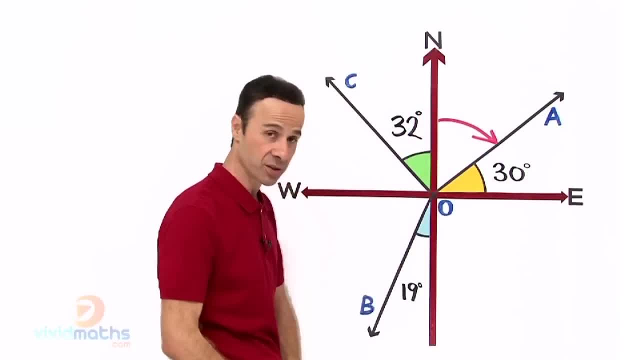 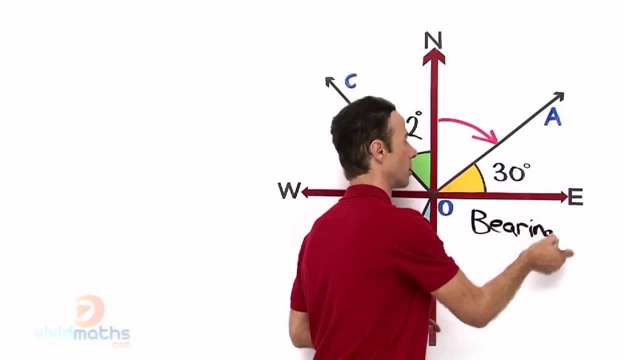 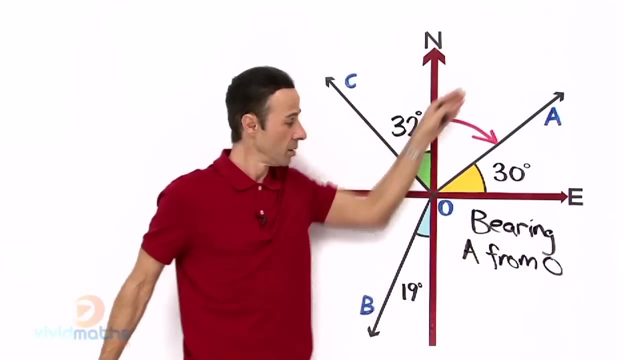 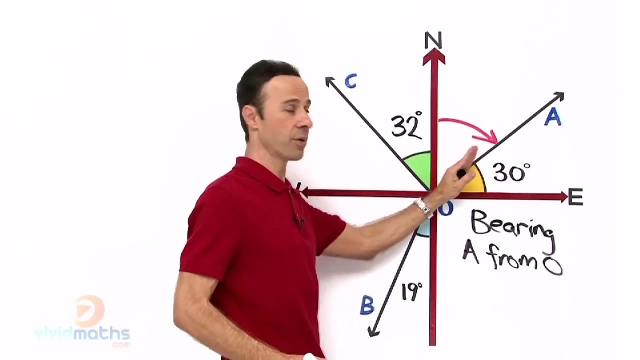 north clockwise. yeah, So let us work this out together. So we have bearing of A from O, bearing of A from O. yeah, That is what we are looking for. that is going to be 90 degrees, take away 30,. yeah. 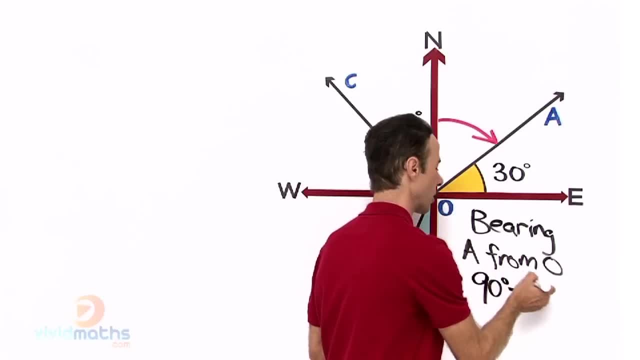 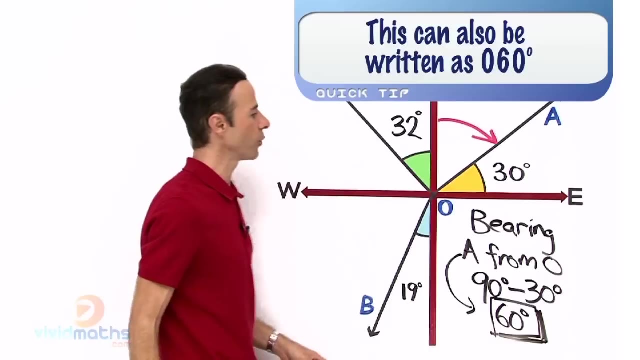 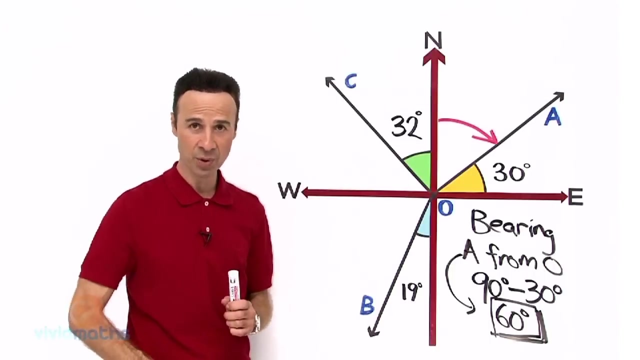 So that is 90 degrees. take away 30 degrees, So the first bearing across there is A A grand total of 60 degrees. there is our first one. okay, let us go for our second one, which is coming down across there. Now, the second one is going to be clockwise. remember, nothing happens without north. 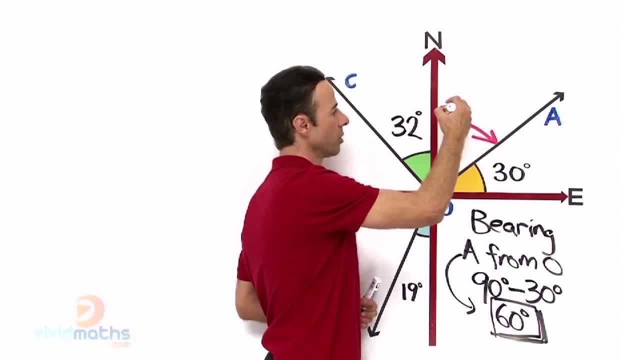 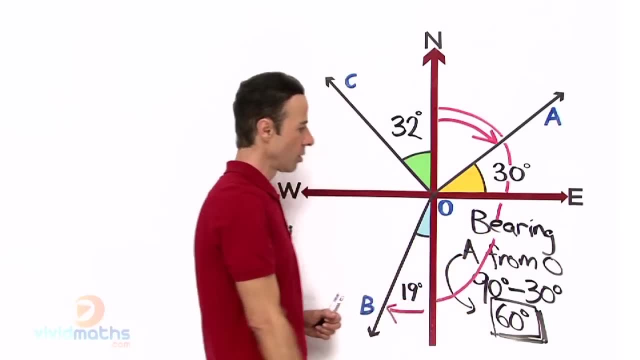 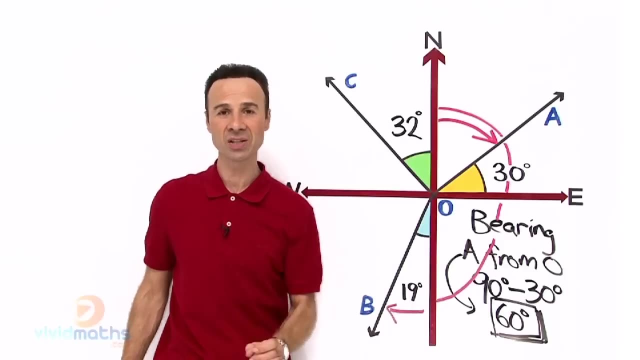 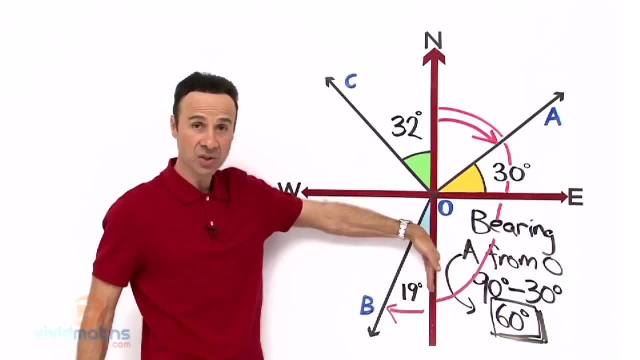 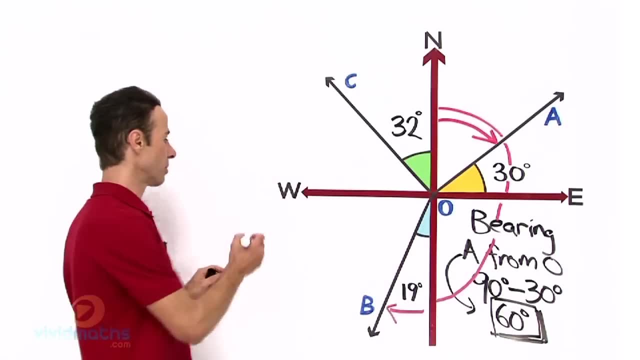 line. all of that sweeps 180 degrees and, as you can see, here we just add that 90 degrees. So let us do that now, let us actually work that out. So for this one here it is going to be the bearing of B from O. yeah. 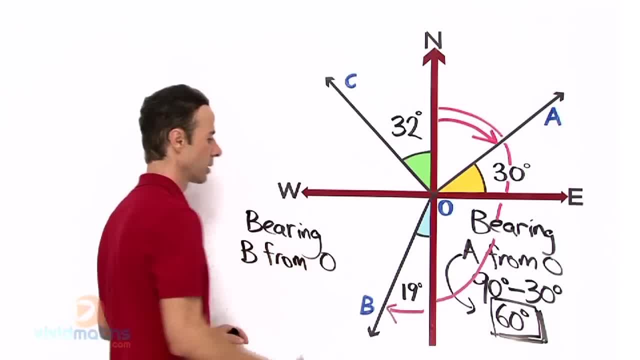 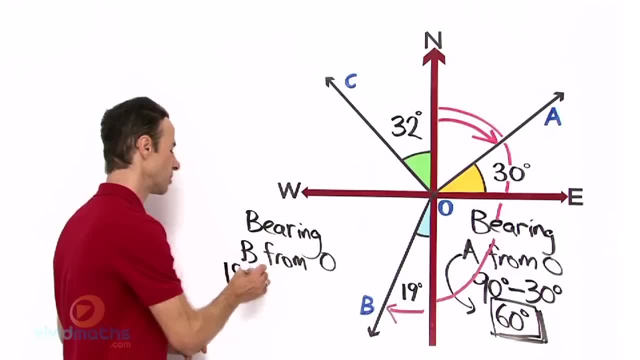 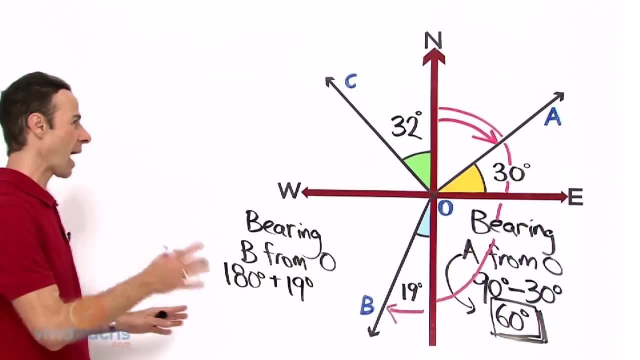 And that is going to be 90 degrees. Okay, So that is going to be, let us see now, all the way around, 180 degrees. 180 degrees then plus the 19, and putting that in your calculator, adding it up together, B from O is going to: 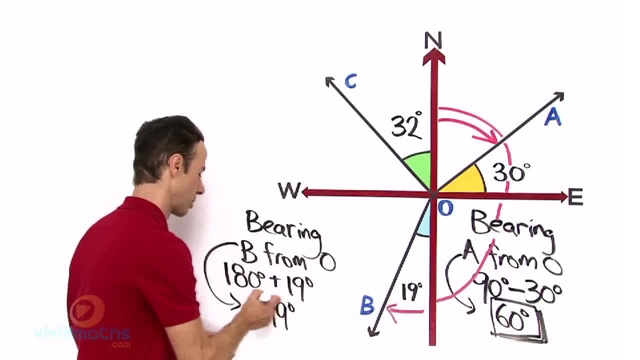 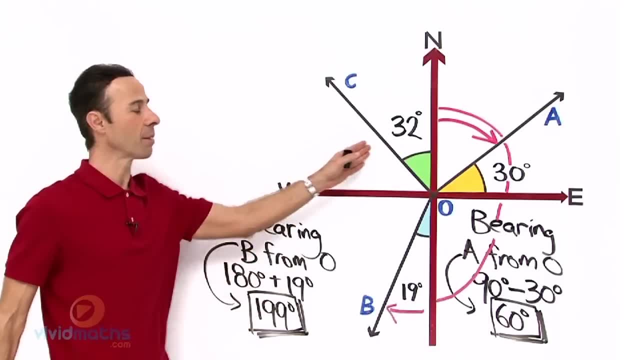 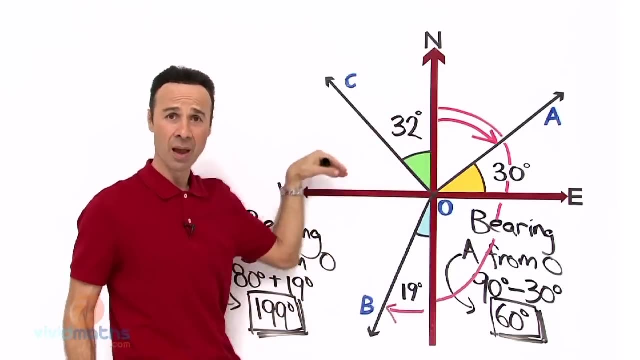 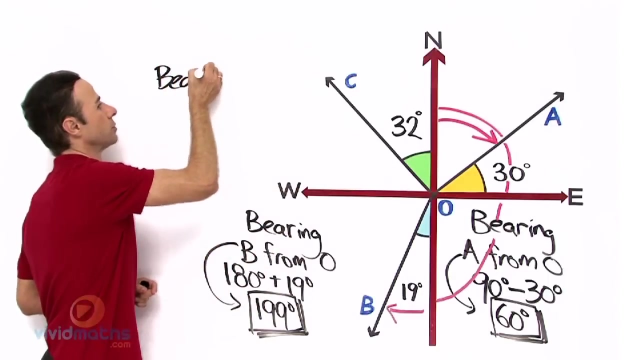 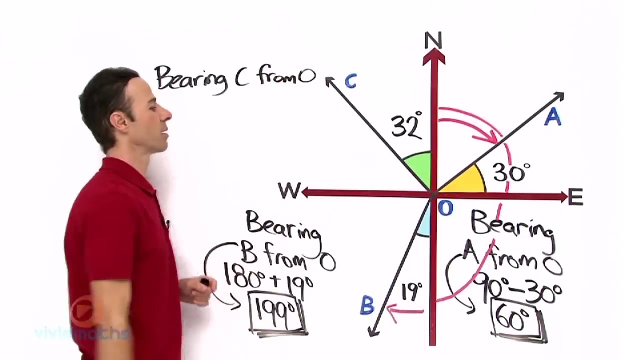 be. there is our second bearing And finally we have the bearing up here. we are going to go all the way around revolution and then take away that 32 gap there and that is going to give us the clockwise bearing from north. So let us have a look here. this is going to be bearing of C from O. let us point that. 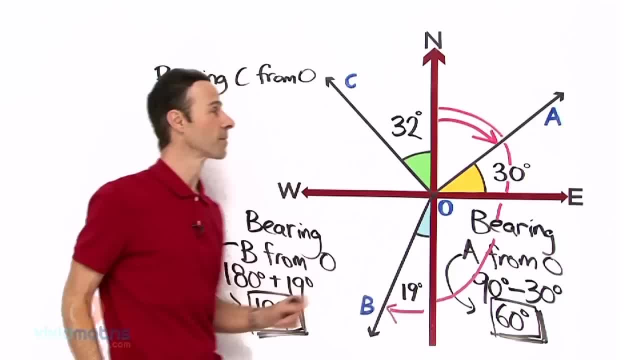 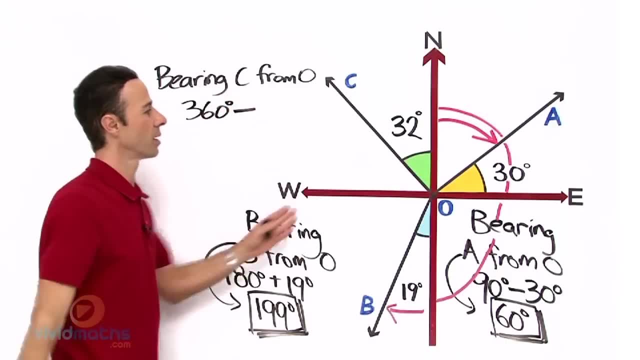 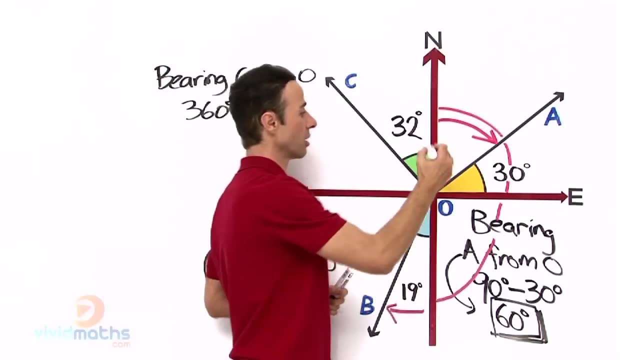